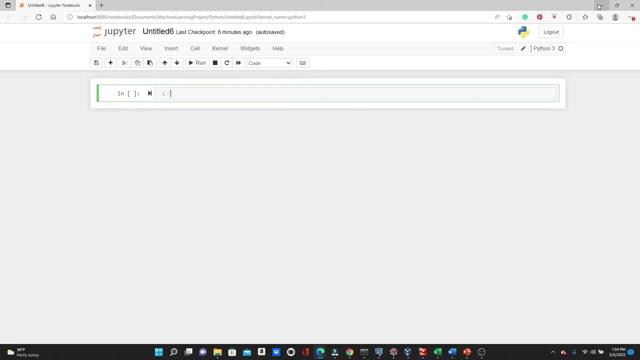 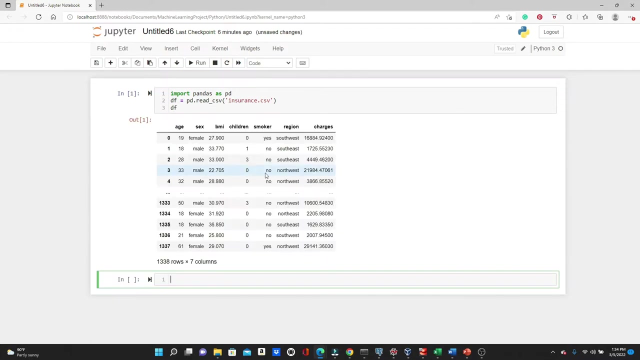 we will use a dataset that almost resembles a real world dataset. Let's see the dataset. first, In the same site, import pandas as pd and now dfpdreadcsv- insurancecsv- df. This is the dataset. I have the link to the dataset in the description box below. Please feel free to. 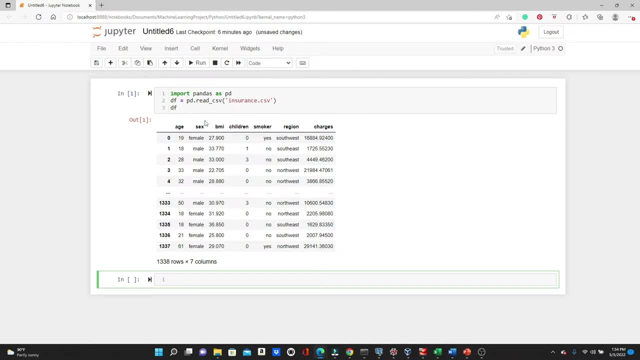 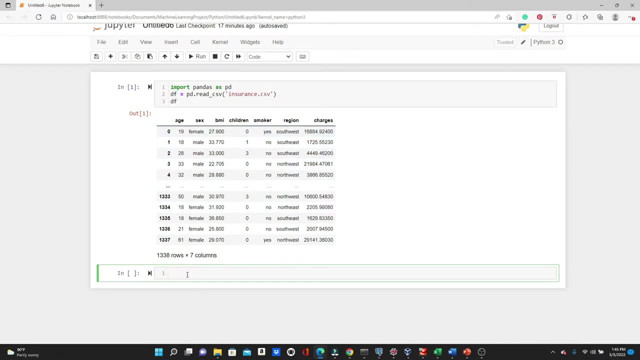 download and follow along. So this is the insurance dataset. We have age, sex, pmi, children. You can use the cpc. they are. these are the percent data set. here. We have age, sex, PMI, children and smoker region and charges. these are our variables. before we can move on, we need to do. 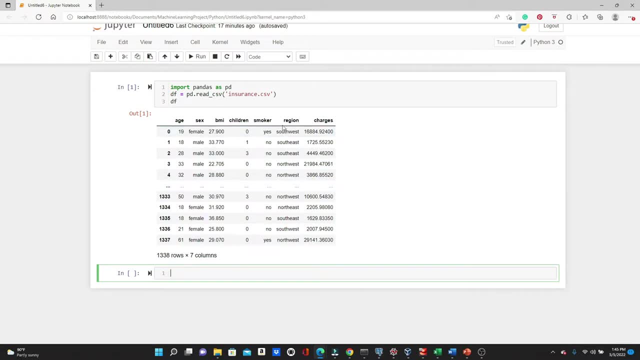 some work on this data set. look, the sex region and smoker are categorical variables and contain string values. we need to convert them to numeric values. so let's do that. start with sex, first. we need to convert it to as type category, and then- and let's convert- 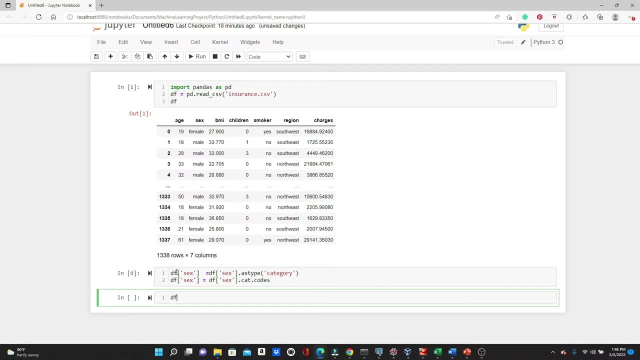 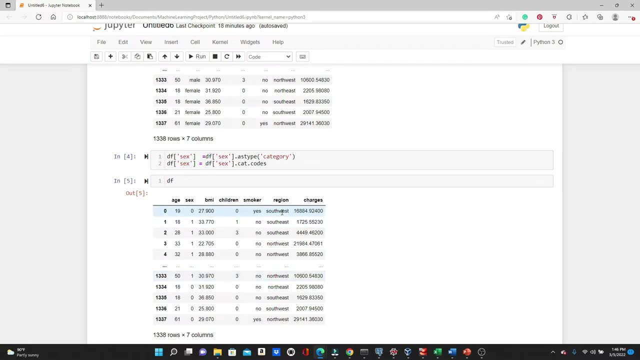 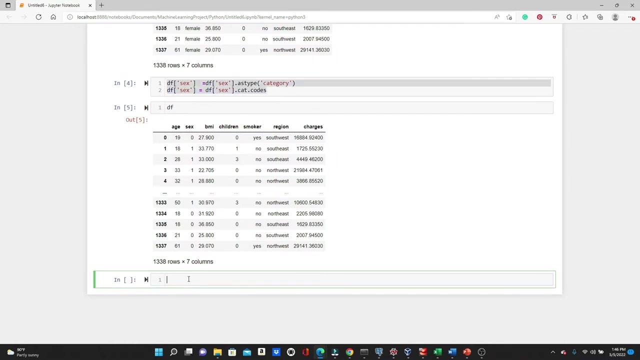 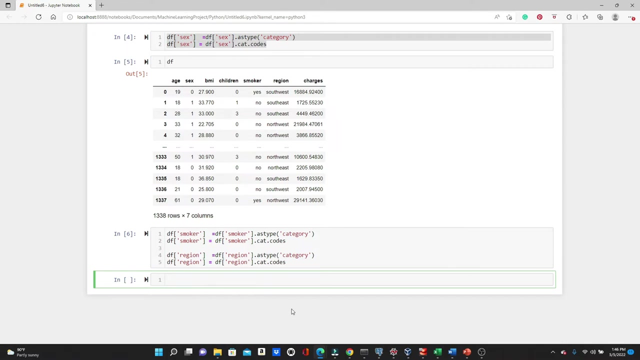 dot cat codes. now let's look at df. now look, instead of male and female, we have zero and one now. so we need to change smoker and region in the same way. let's copy them and paste. so let's look at the dfs. look, all of them are numeric now. now we need to check if any of these 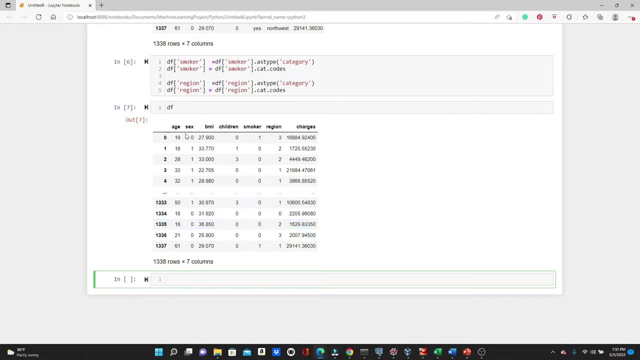 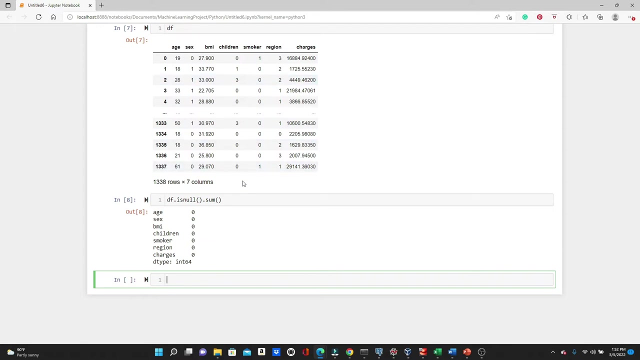 columns contain any null values. df dot is null, dot sum: look, there is no null values, so the data set is totally ready for the modeling. now let's go ahead and do some work on the dfs. what is the task today? the task today is using all these variables and predicting the charges. 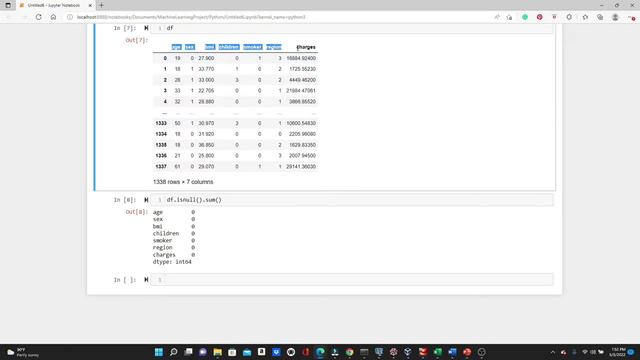 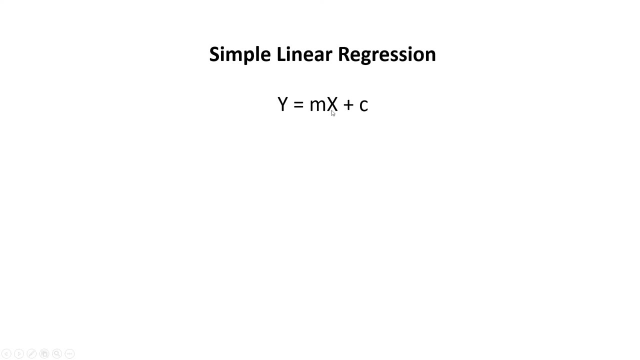 so these variables are the training features and charges will be our labels. in our last video we have seen that this is our linear regression formula: y equals to mx plus c, where x is the training feature and y is the label. so we have only one training feature and one label. 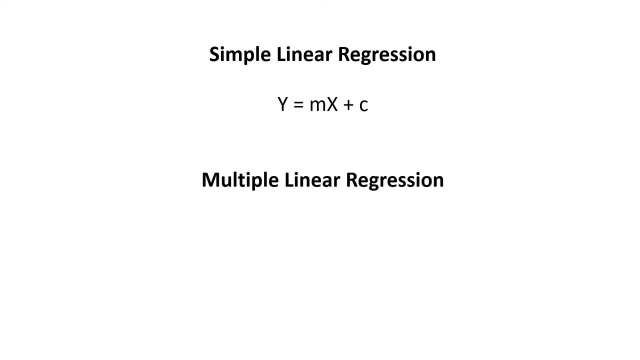 what happens when we have several training feature. so in multiple linear regression we have several training feature, right? so instead of x, we will have x1, x2, x3, all the way up to xn. instead of m, we will have m1, m2, m3, all the way up to mm, and the formula will become like this: m1, x1 plus m2, x2. 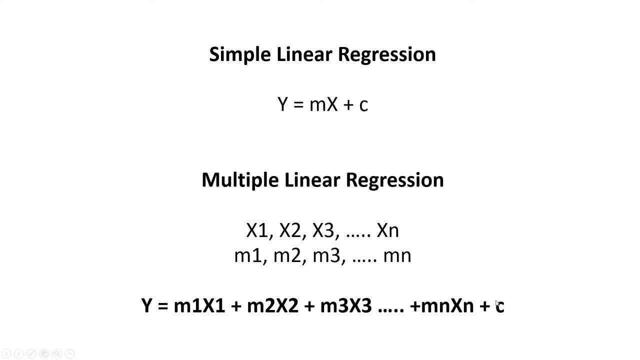 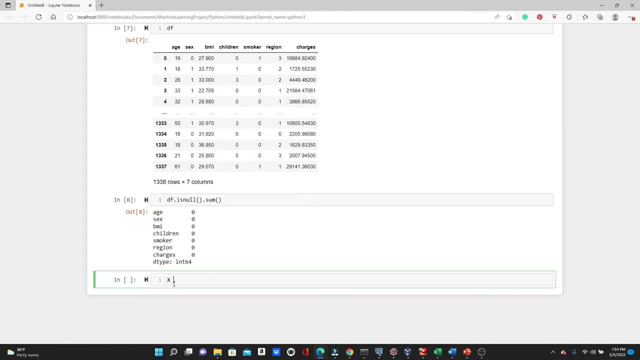 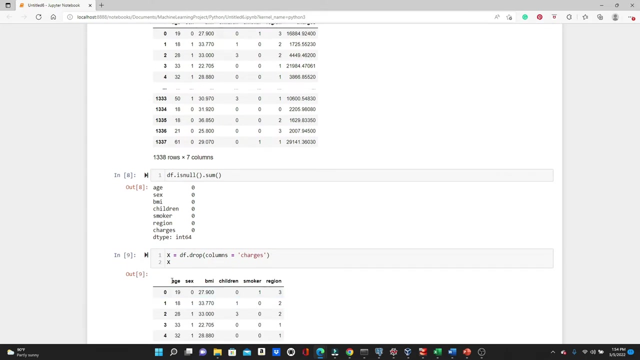 all the way up to m and xn plus y, intercept, as we already mentioned. the formula will be like this: as we already mentioned before, these are our training features. so let's define the training features: df, dot, drop columns, columns, charges. so this is our training features. look, the training features we 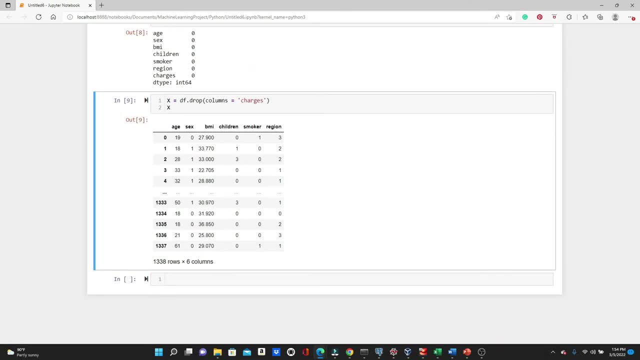 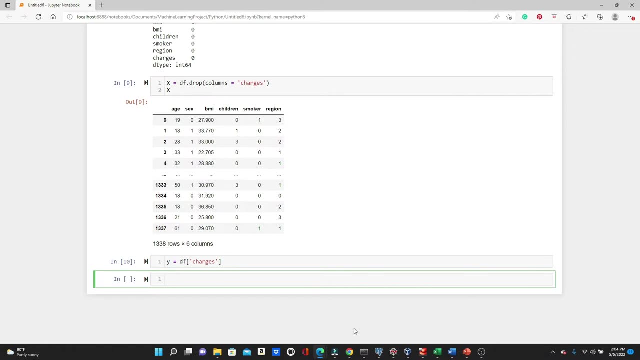 have all the variables except the charges and our label. our label is df charges. the next step is to split the data set so that we can keep portion of the data set for the training and portion of the data set for the testing. for that we are going to use train test split method. 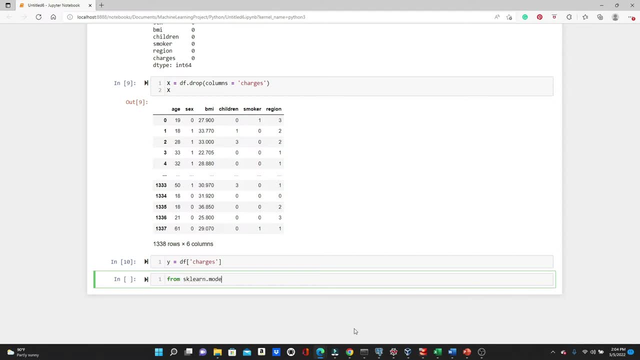 from the scikit-learn library: dot model selection: import train test split. okay, now x train x test. not this way: x train x test, y train y test. then i would use this train test split method. we will pass our x, y and test size 0.3. so test size 0.3 means this will keep 30 percent of the data for the. 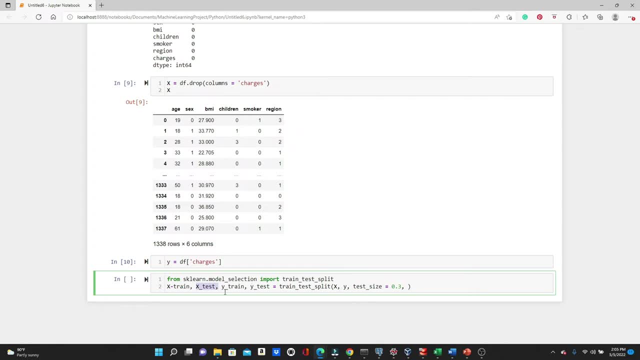 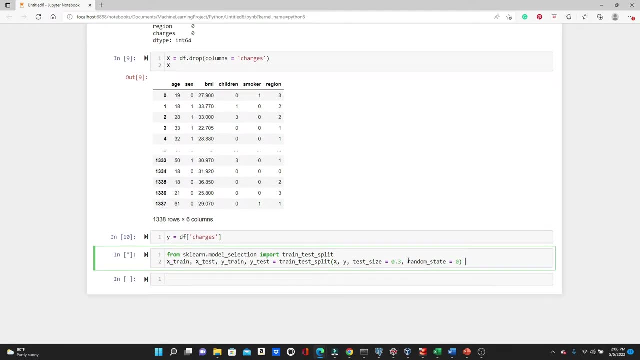 testing as x test and y test and 70 percent of the data for training. then random state 0.. the random state will help you recreate the same train test, split if necessary. we are ready for our machine learning model now. so first we will import the linear regression from sp learn. 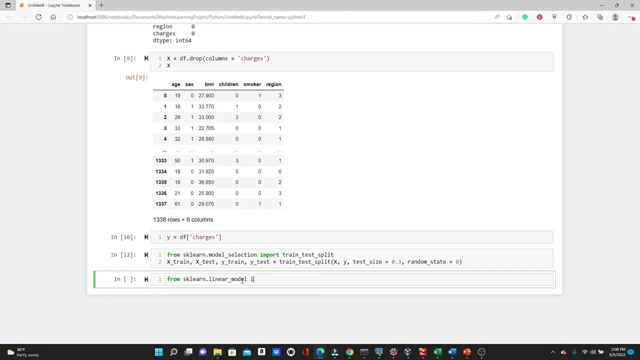 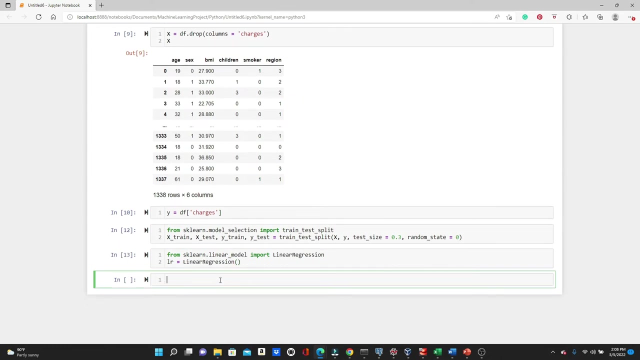 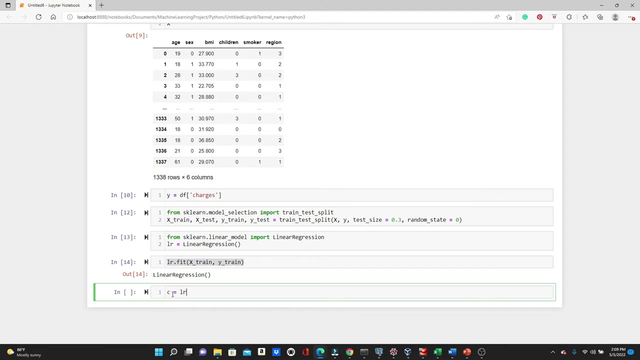 dot linear model- import linear regression. okay, now we will save the linear regression model to this variable nr. then let's fit our training data to the linear regression model. x train- sorry, y train. yeah, the model should be trained now. so let's see the parameter first. see the y intercept: l r dot intercept. 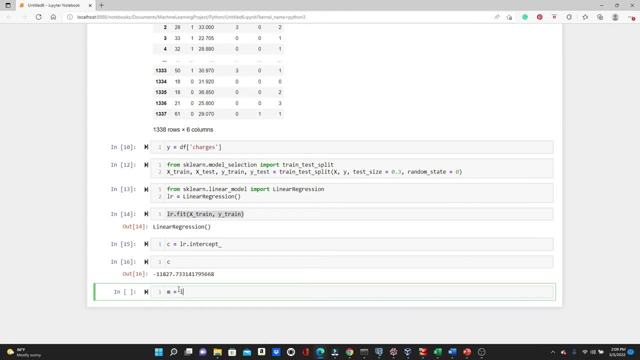 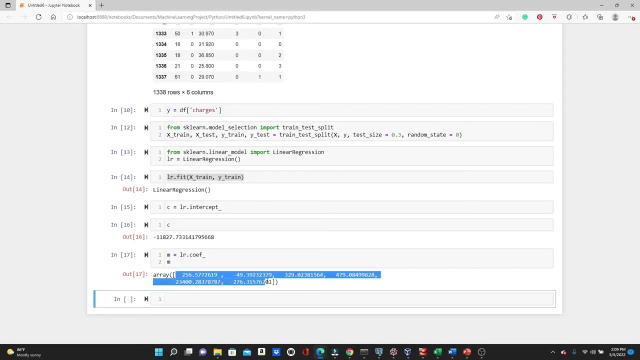 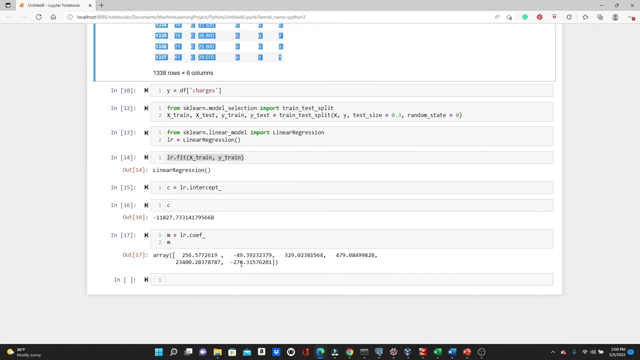 this is the y intercept and m l r dot 12. that is coefficient m. you can see we have six coefficients for our six training features. so we have six training features. so we got our six coefficients. the model training is done. the training part is done. now we need to see if the model is actually working. 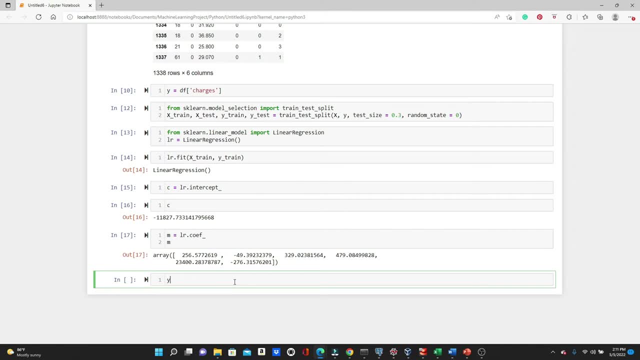 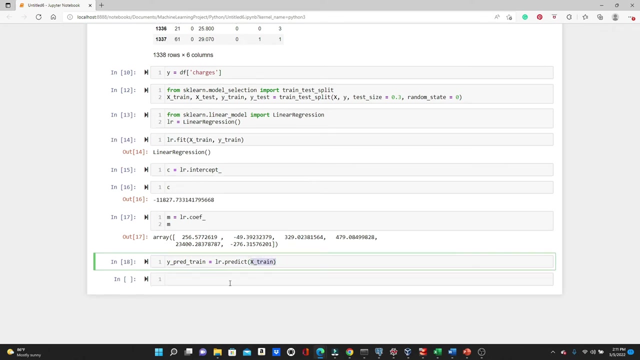 let's try to predict the charges using the training set y crad crane. lr dot predict. so we are going to use the predict method and we will pass x train. it should predict the charges for this x train data now y crad train. so yeah, that's fine. 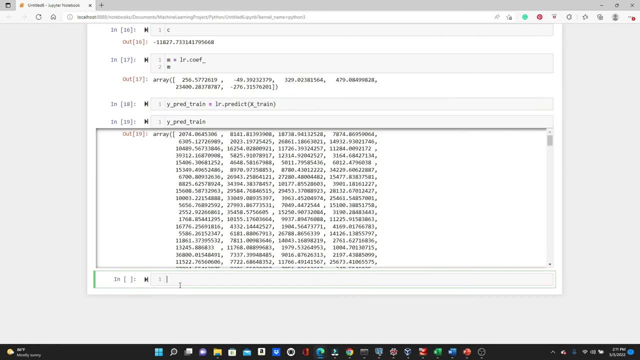 So yeah, the prediction is done. but how good is the prediction? Let's check Import matplotlibpineplot as plt, pltgetter, ytrain and yprettrain. So if we put this x train in the x direction and this x prettrain in the y direction, 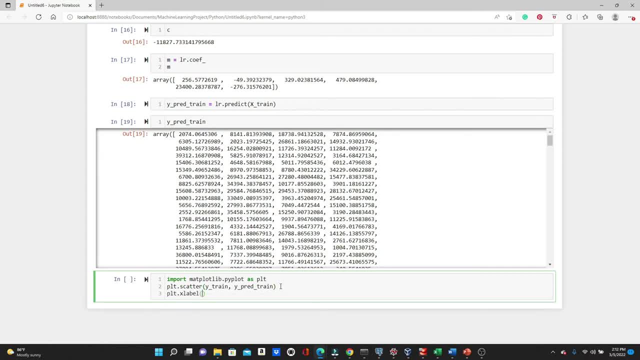 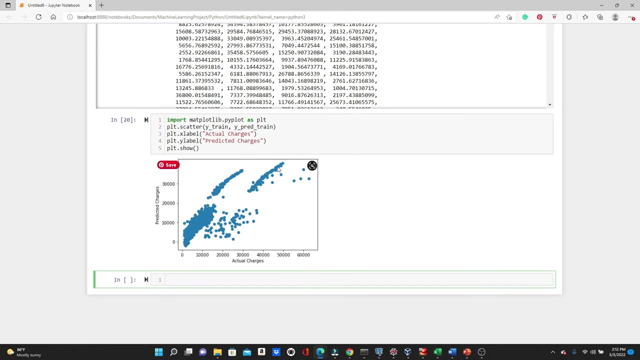 we will actually see how good is the prediction in terms of visualization, Actual charges and plty label is going to be our predicted charges. So pltshow For some of the data prediction looks pretty good here and here, but for some of the data 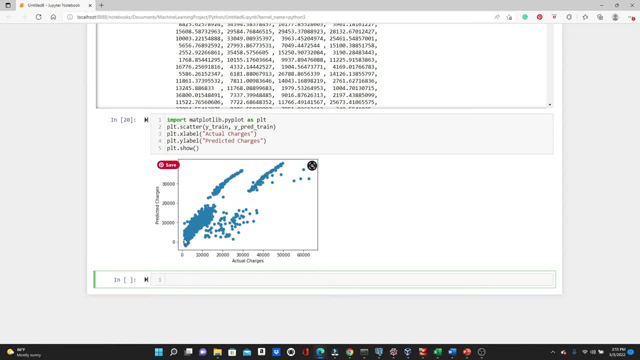 it looks very bad. It looks very sparse. How do we know how much prediction is good and how much prediction is actually not that good? We can use r-square value or r2 score. So we have to import r2 score from sklearnmetrics. 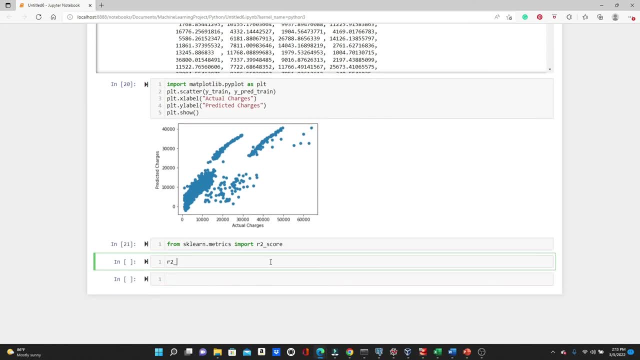 Import r2 score. So r2 score: We need to pass ytrain and yprettrain, So 73.. This is the r2 score. What r2 score does it shows you how close the data have fitted to the regression line. 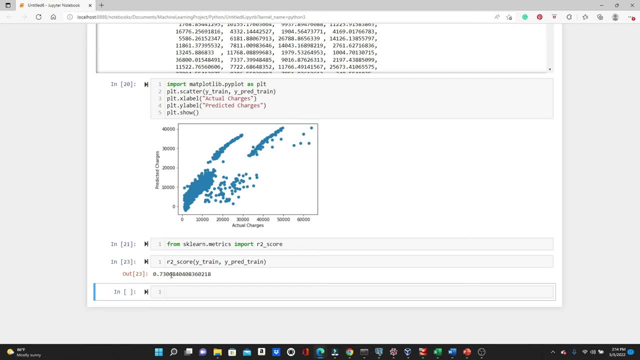 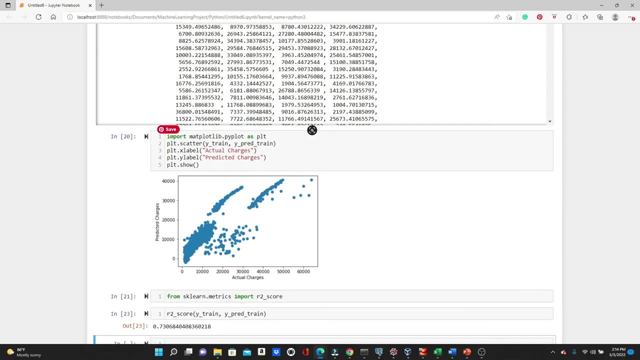 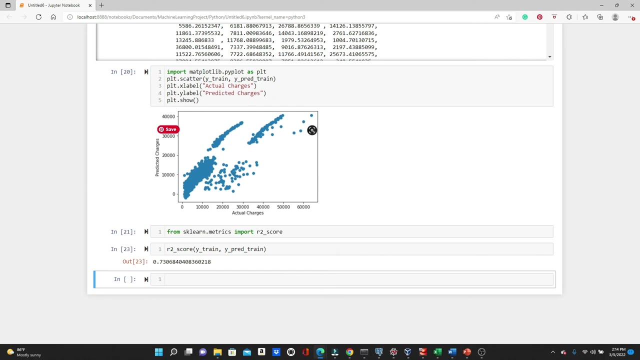 or the portion of the variance for a dependent variable. that means the charges can be explained by the independent variables in the regression model And the independent variables are our training features. What portion of the variance in the charges can be explained by our training features? 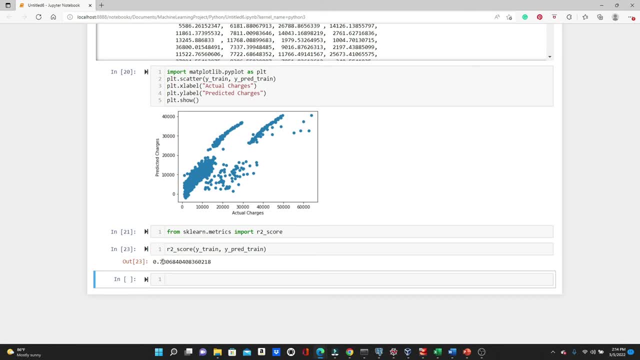 So 73.. So this is 0.73.. So r2 score can be from 0 to 1.. If the r2 score is closer to 1, that means model is better. If the r2 score is closer to 0, that means model is really bad. 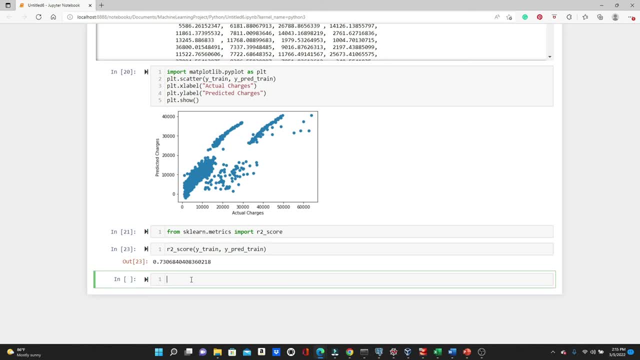 So it's 0.3.. It's actually closer to 1.. So we can say that the model is acceptable. It can be further improved. There are several ways we can try to improve our model, but we will talk about it in some. 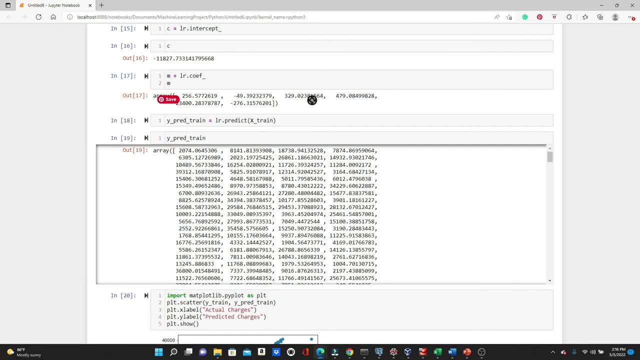 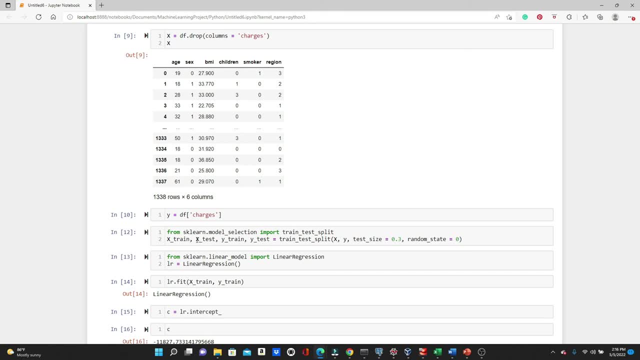 later video. So all this time we evaluated the model, We will use the training data And we also use the training data to train the model. We will know how the model is working actually when we will use the testing data, because our model never have seen the testing data.